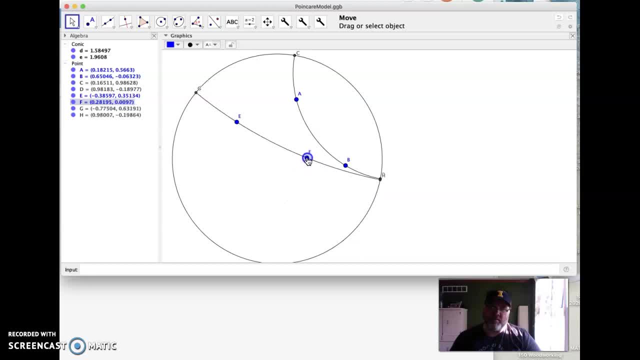 Notice as I drag it, I haven't intersected, I haven't intersected, I don't intersect until this point H, down here, gets on, aligns with D, So I'm you know, we get there, and then all there, it finally intersected, Finally intersected. So, but all through here the line is not intersecting. There's no, and so what does that mean? about parallelism? That must mean that there's a lot of lines that are parallel. If we define 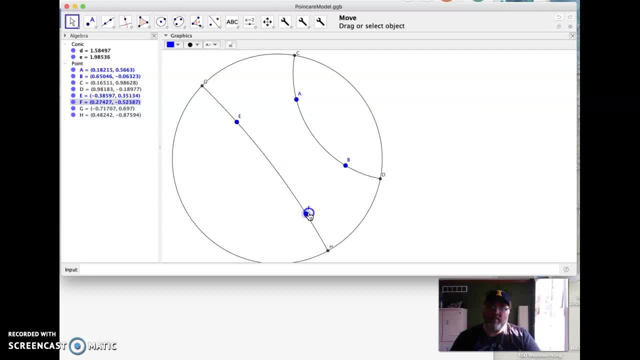 parallelism to be two lines, parallel lines to be two lines that don't intersect, So this line doesn't intersect, that line doesn't intersect, etc. Now they're going to also want us to do a construction where we construct two lines, we construct that one. My bad, Back it up. We construct this line here And we construct this line there. 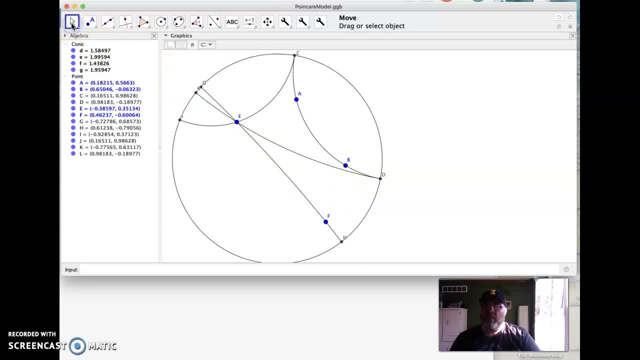 And what you'll notice is that if I grab and drag this line, that it's like a boundary, This line won't intersect a- B until I get to right there, And then it intersects Once it crosses that boundary there, And then then I've got an intersection. Same is true over here. I got to swing it around, But once I cross that, then the line intersects on the other side, And what these are called are limiting lines. Yeah, this is a good way to do thatf. you want to use this? That's a good thing. Yeah, So I'm going to. 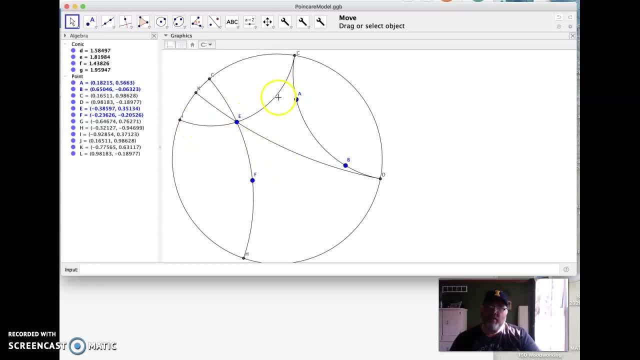 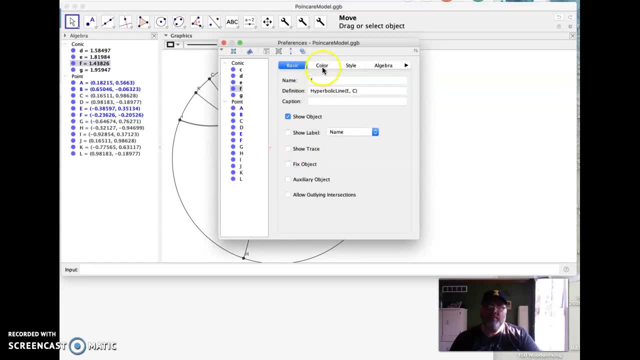 parallel rays. so this ray here- and perhaps I could, we can make it. um, let's see if we can do. let's make it red and maybe we can make it super thick. okay, that'll work. so that line there. and then let's do this one here, let's make it. 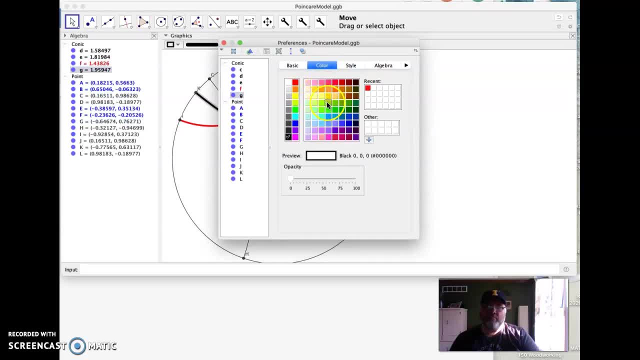 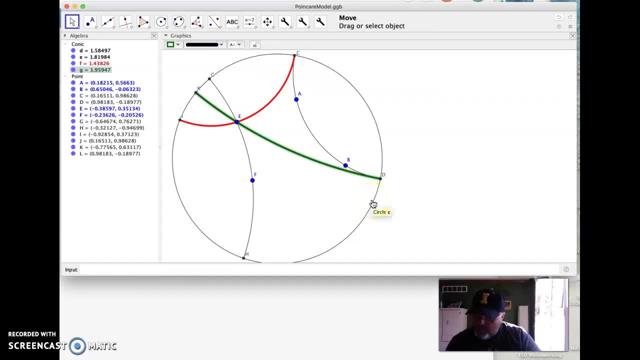 super thick and let's make it mmm green. so those are what are called limiting parallel rays and that means that as out as long as this line isn't getting across those pair limiting parallel rays, it's not intersecting with this other line that we're interested in. okay,